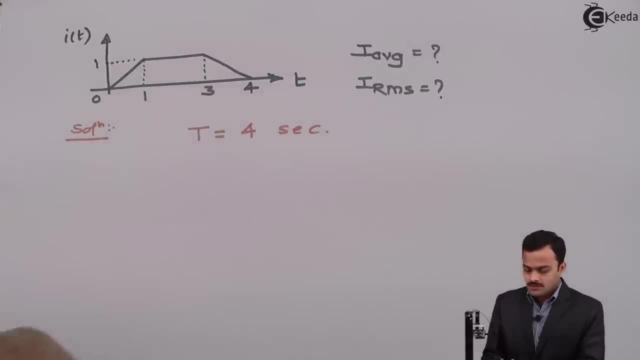 it is changing its shape several times. So from 0 to 1, it is a straight line passing from origin with a some slope. From 1 to 3, it is a straight line of having a slope 0 and a constant value of 1. and from 3 to 4, it is a decreasing slope. 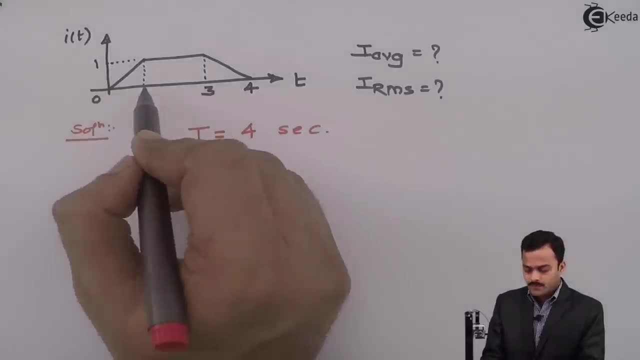 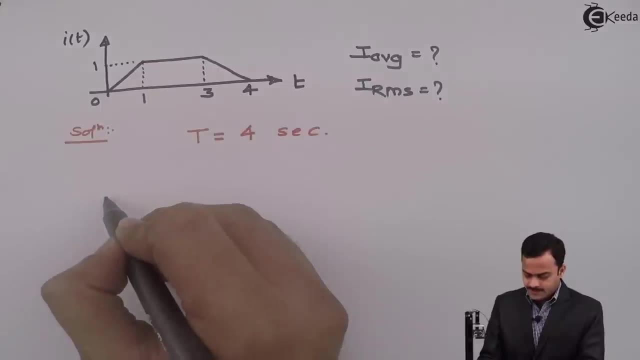 We need to find out equations from 0 to 1, 1 to 3 and 3 to 4.. So from 0 to 1, it is a straight line like this, and there are two points whose coordinates are 0, 0 and 1, 1.. 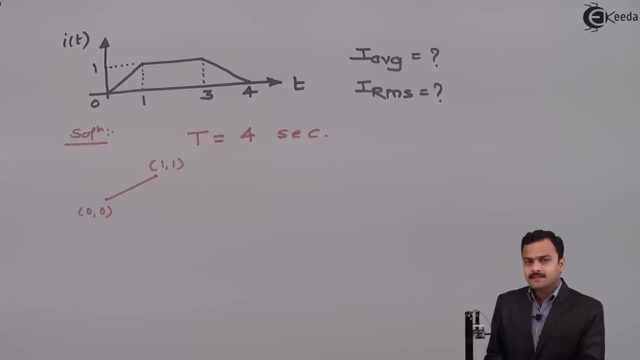 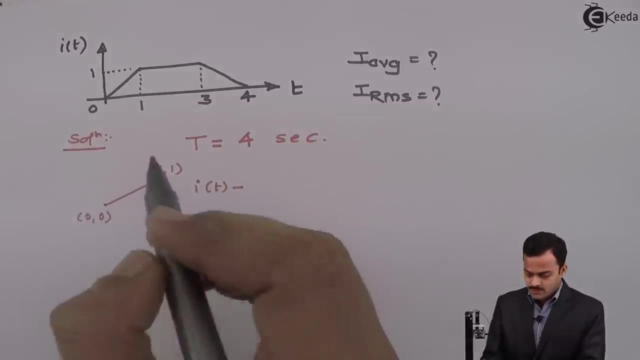 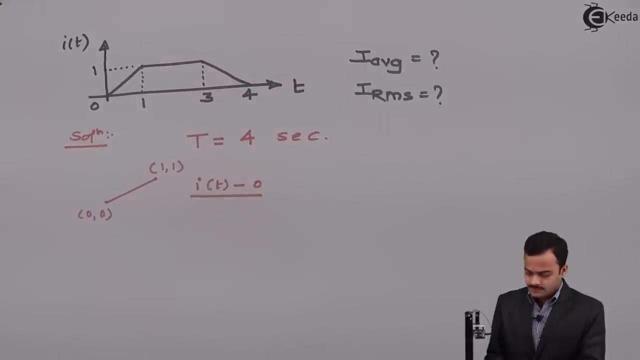 So let's write equation of a straight line: So y minus y1.. So y is I of t. y1 is 0 upon x minus x1.. So x is t. x1 is 0, again equal to y1 minus y2.. So it is 0 minus 1 upon x1 minus x2, 0 minus 1.. So if I simplify, 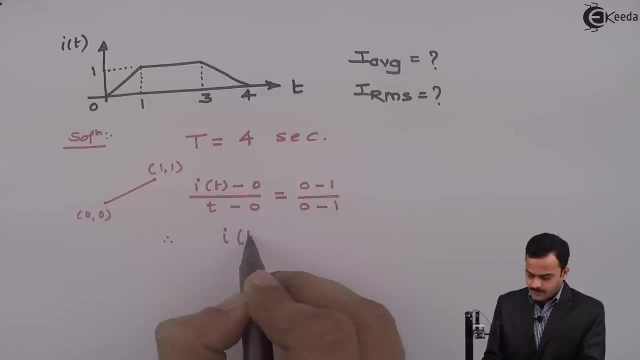 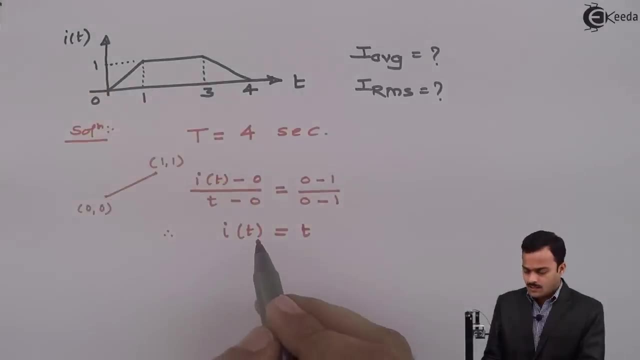 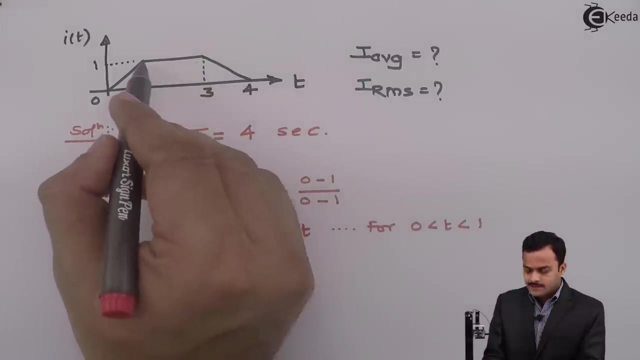 this what I will get: I of t equal to t. So current will have a equation: I of t equal to t for t greater than 0, less than 1.. Second part: it is remaining same, having a value 1 between 1 and 3.. 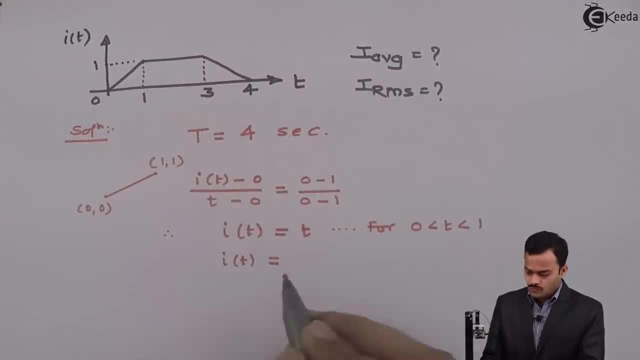 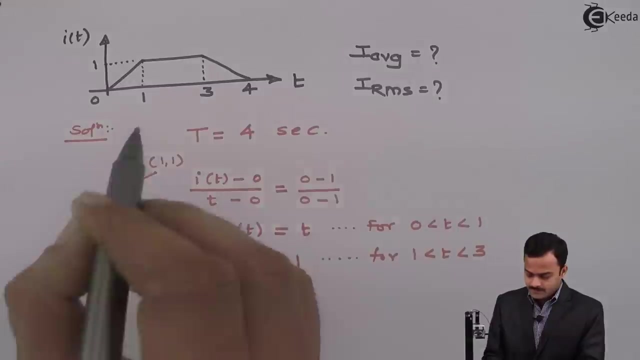 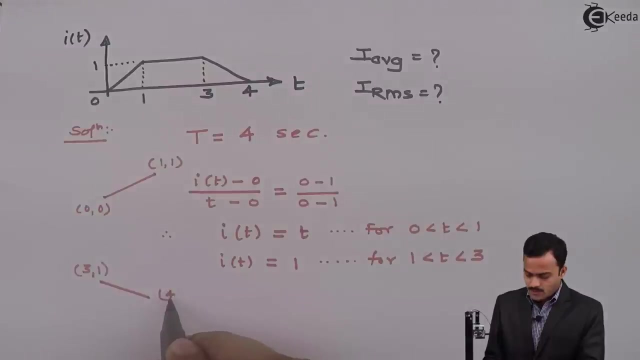 Similarly I of t equal to 1 for t greater than 1, less than 3, and third part, it is a decreasing slope like this. So again there are two points whose coordinates are 3, 1, comma 1 and 2, 0 into 0. So t equal to 1, whole root of 1, will be 0. So in this case 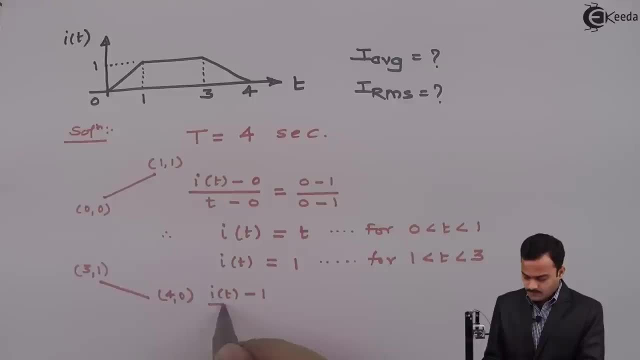 we cannot write a equation of a straight line. So say: if I just write an equation of a straight line, y1 minus y2 upon x, minus x1 equal to y1, minus y1 upon x1, minus y2 upon x1 equal to y2 prior, What do I do? I just write a equation from that square which gives: 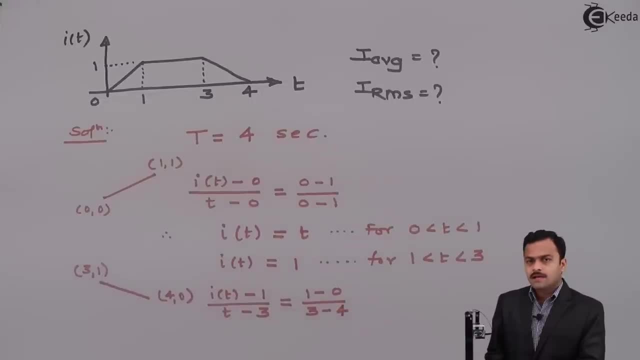 the ratio y2, violenta y1 divided by x, So it is r to the power minus grams times x1, x1 minus x2.. So I am getting this equation i of t minus 1 upon t minus 3 equal to 1 minus. 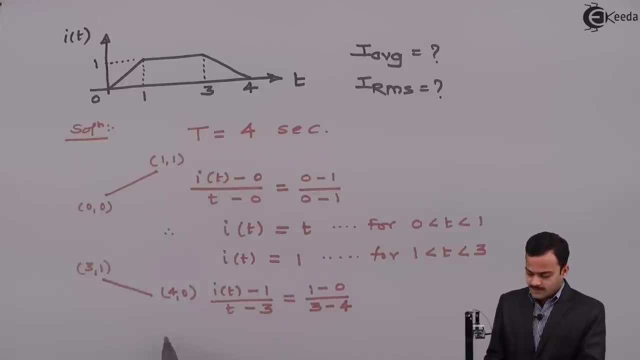 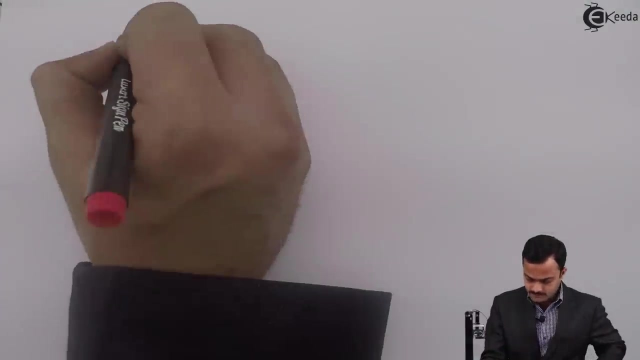 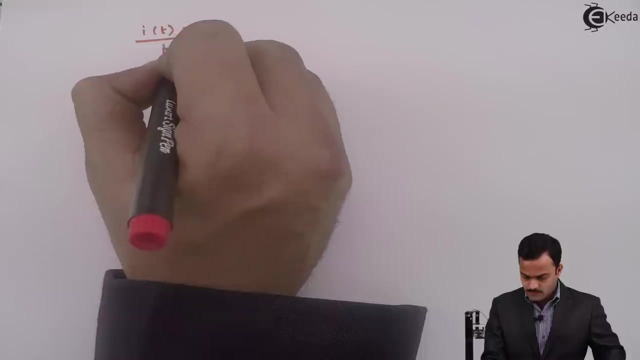 0 upon 3 minus 4.. So let us simplify. So what I will get? i of t minus 1 upon t minus 3, equal to 1 upon minus 1.. So if I simplify further, I will get i of t minus 1 upon t. 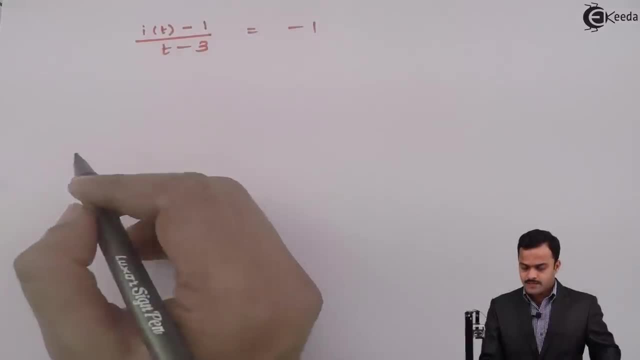 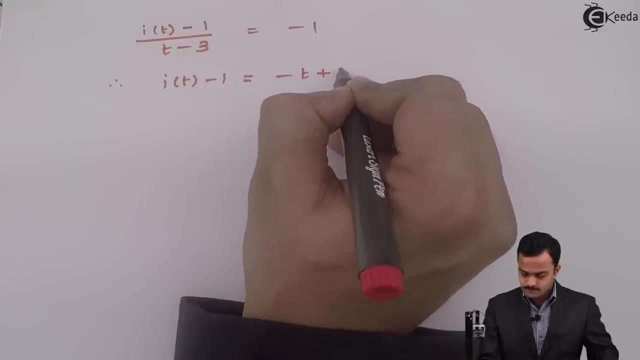 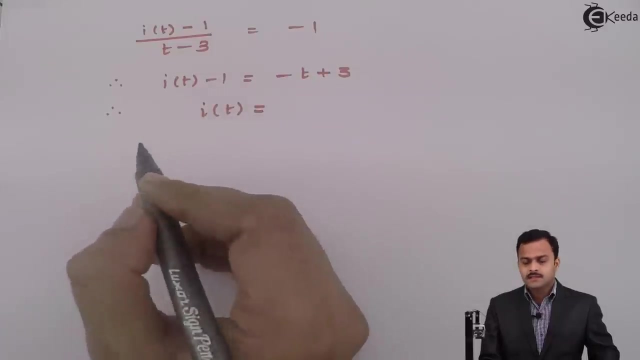 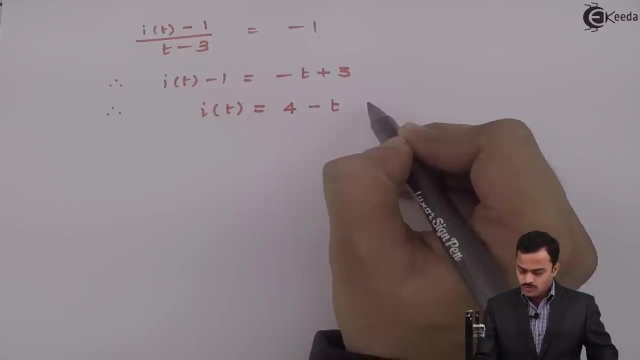 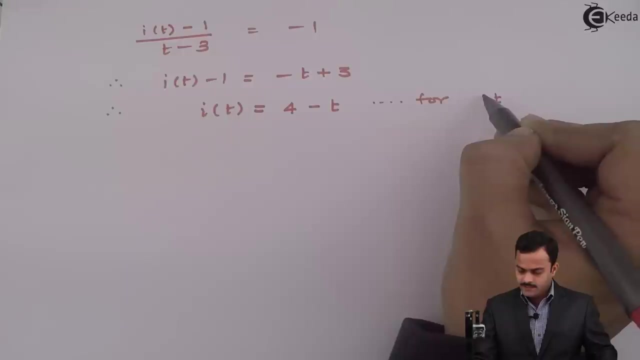 minus 3, equal to minus 1.. If I cross multiply, I will get this equation Which, further simplifying, will give you i of t equal to 4 minus t. So current waveform will have this equation for t greater than 3, less than 4.. So now, in the time period, 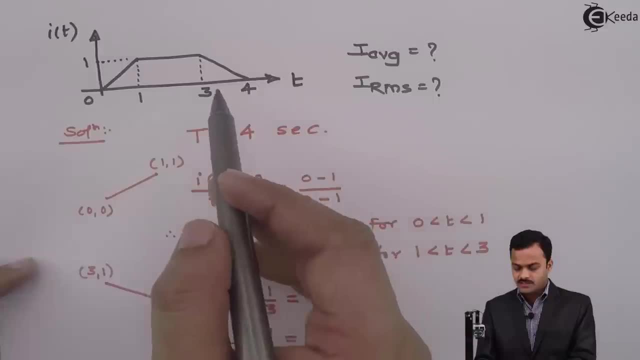 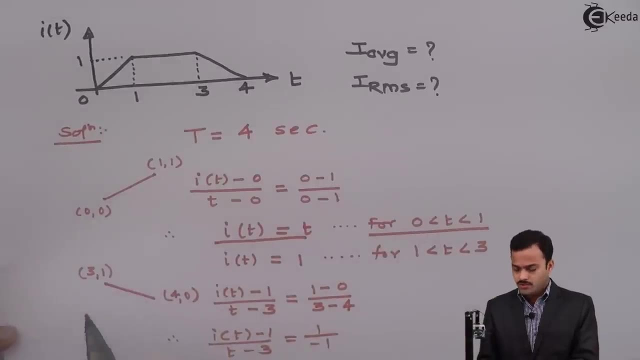 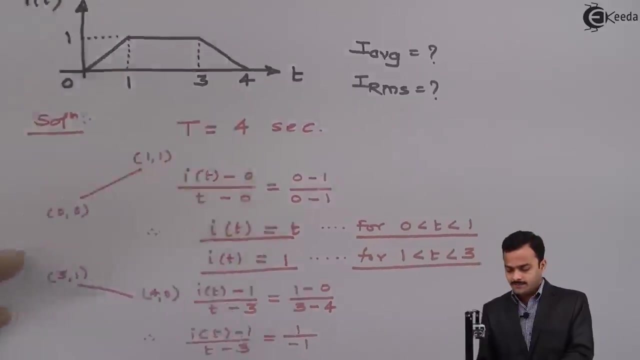 number of times. So current waveform is changing. it is equation, So this current waveform is changing its equation. We have written i of t, equal to t for t between 0 and 1.. It is constant, which is equal to 1 for t between 1 and 3.. 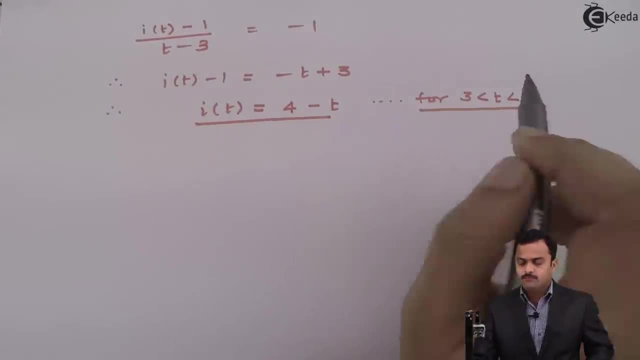 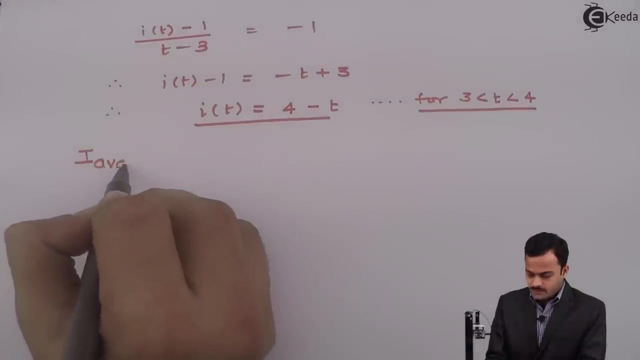 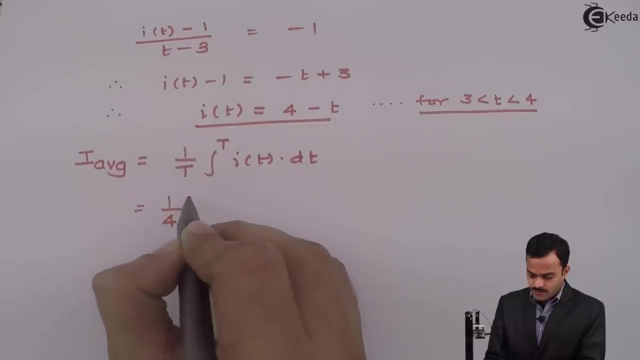 i of t is 4 minus t for t between 3 and 4.. So let us write the equation of the averaged value 14″, Which is nothing but 14″, 14″, 4″, 1 over time period t. we have to integrate I in the time period t, So it is 1 by 4 and 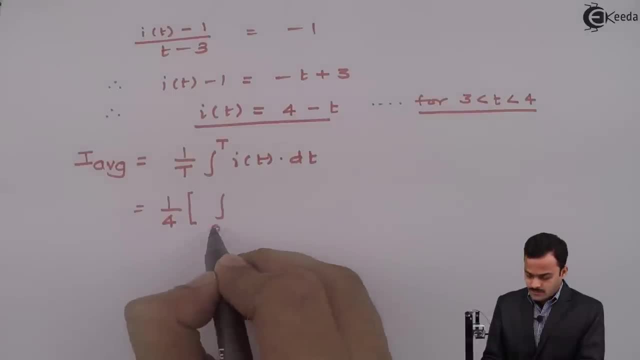 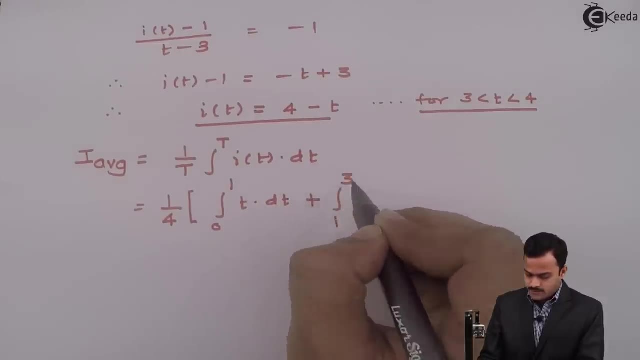 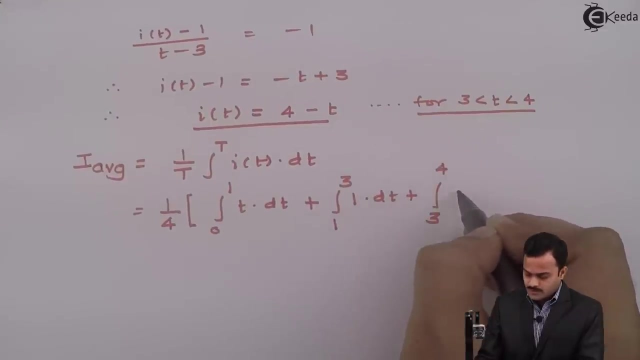 this time I am having three parts of equation: 0 to 1, it is t plus 1. to 3, it is constant 1, and from 3 to 4, it is 4 minus t. So if I solve I will get t. square by 2 is the integration. 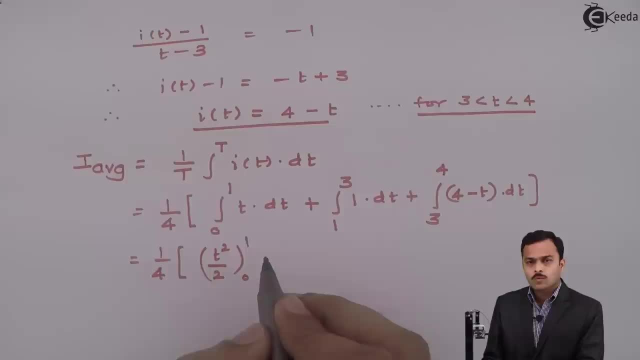 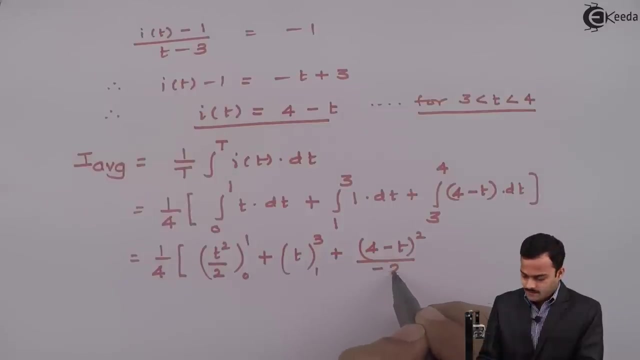 of t limits 0 to 1, constant integration is t limit 1 to 3.. And here the integration is 4 minus t, the whole square divided by minus 2, and limits are 3 to 4.. So if I apply the limits, what I will get? 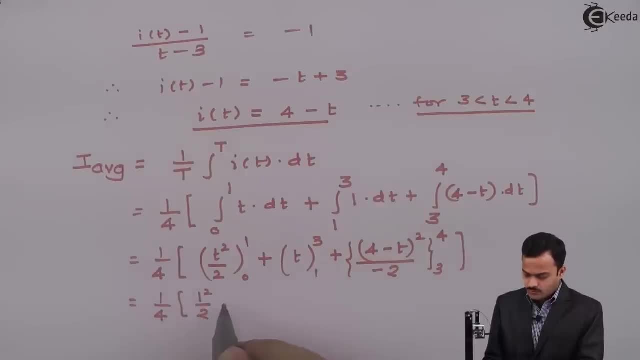 1. 1 square by 2 minus 0 plus 3 minus 1 minus 1 by 2, I will take out, because it is a constant and if I apply the limits, what I will get: 0 square minus 4 minus 3, the whole square. 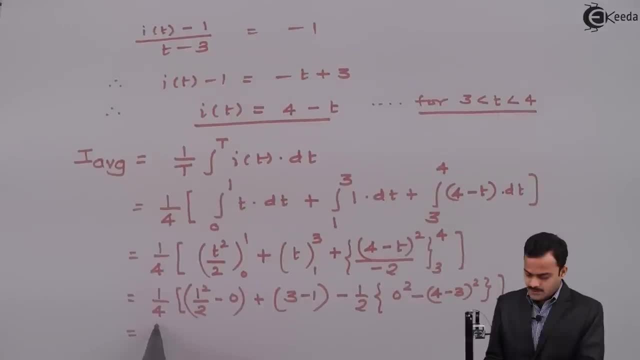 So ultimately it is 1 by 4 and bracket 1 by 2 plus 2.. Here, 4 minus 3 is 1, 1 square is 1, this minus, this minus will become plus, So it will be 3 by 4.. So it is 1 by 2 minus. 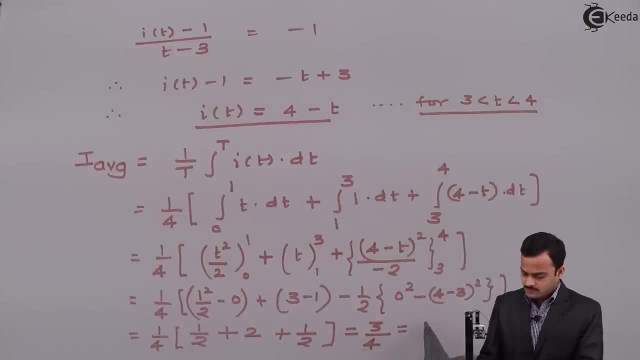 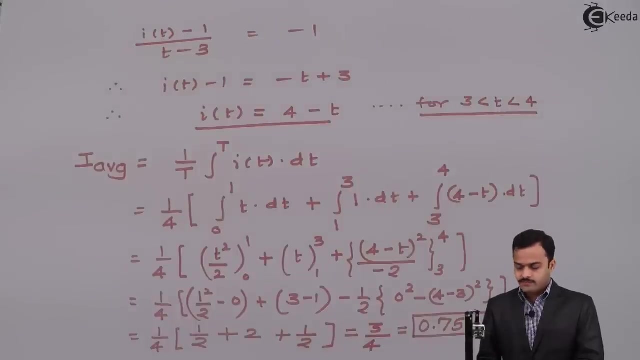 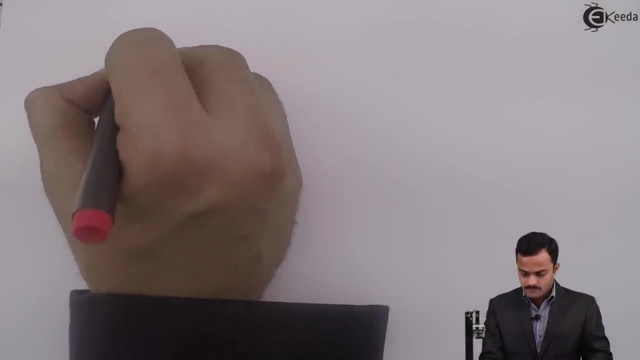 3 by 4, which is nothing but 0.75 ampere. So the answer here for average value is 0.75 ampere. Let us solve it for RMS value. So I RMS is root of 0.75 ampere, So I RMS is. 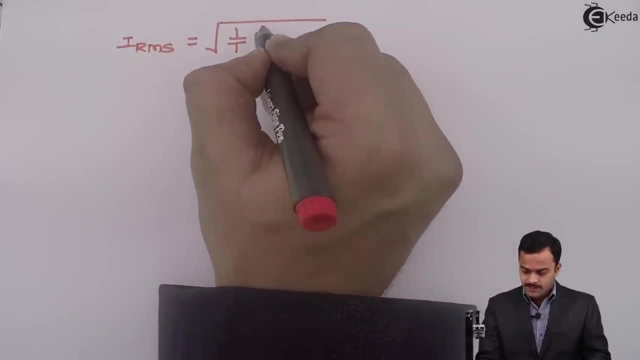 0.75 ampere. So I RMS is root of 0.75 ampere. So I RMS is root of 0.75 ampere. So I RMS is 0.75 ampere. So I RMS is 1 by t. integration over a complete time period. t I square dt. 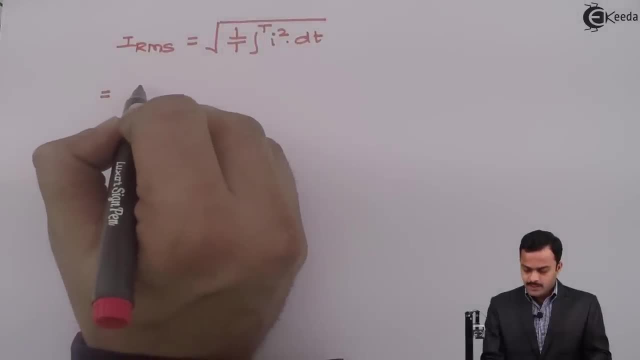 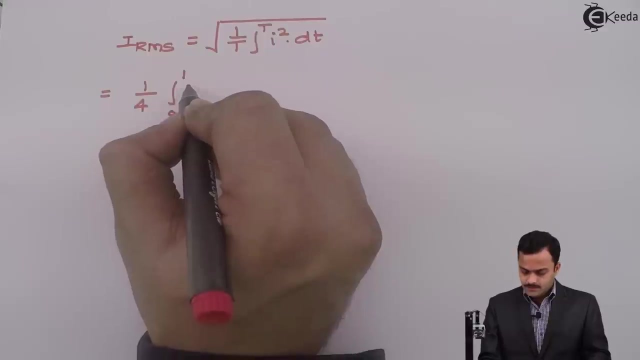 So it will be 1 by 4.. Integral have 3 parts. one is from 0 to 1, where I is t. So t is 1 by 2 minus 1 by 4.. So it will be 1 by 2 minus 1 by 4.. So it will be 1 by 3. So 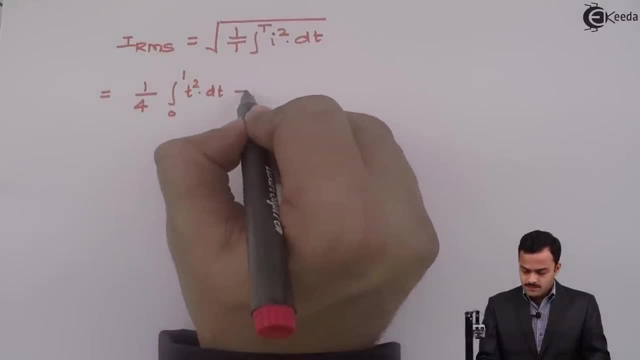 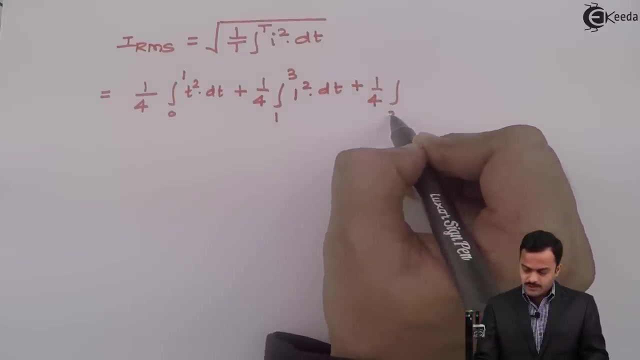 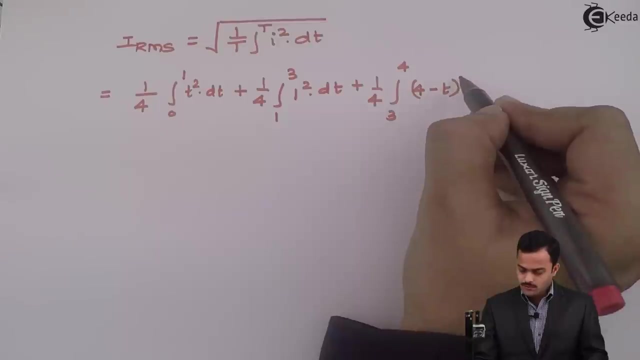 t square dt. second part is from 1 to 3, 1 square tt and third part from 3 to 4, it is 4 minus t, the whole square dt and ultimately we have to take root of this. So raise to. 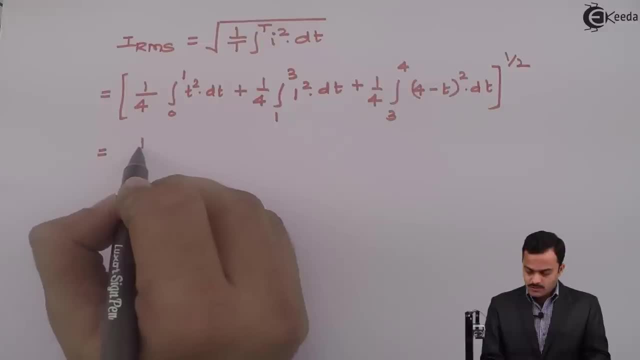 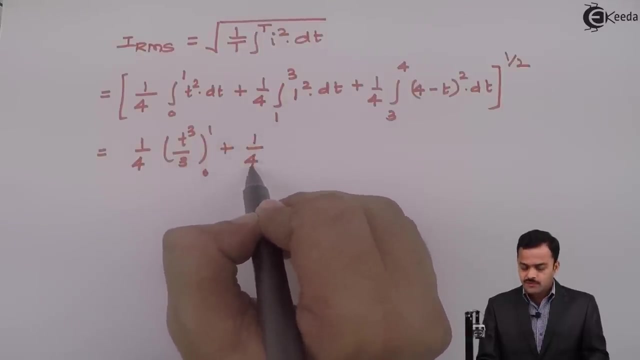 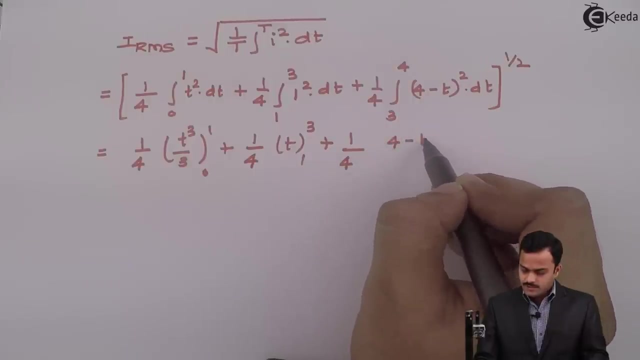 1 by 2.. So if I solve integration of t square is t cube by 3, limits are 0 to 1, here it is a constant only, And integration of constant is t limits 1 to 3, here again the integration is 4 minus. 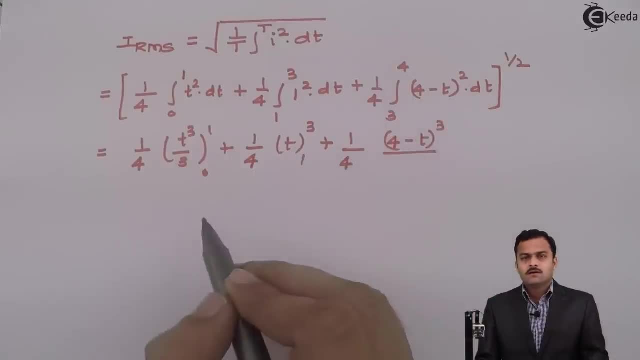 t, the whole cube divided by minus 3, and limits are 3 to 4.. So So ultimately we have to take root of it. So if I apply the limits, what I will get? 1 by 12 into 1 cube plus 1 by 4 inti, 4 minus 1, minus 1 by 12. if I apply the limits, what? 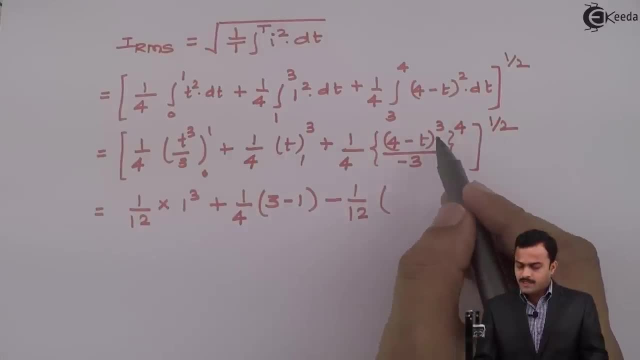 I will get- 3 by 12. shore: If I apply upper limit, 4 minus 4 is 0, so 0 cube is 0, minus lower limit is 3.. If I apply, 4 minus 3 is 1, 1 cube.